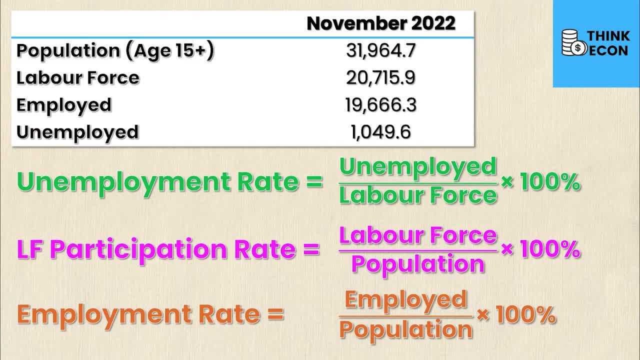 population. Now it's important to note that the denominator of the unemployment rate is the number of people in the labor force, but the denominator of the employment rate is the total number of of people in the working age population, And so, therefore, the unemployment rate plus the 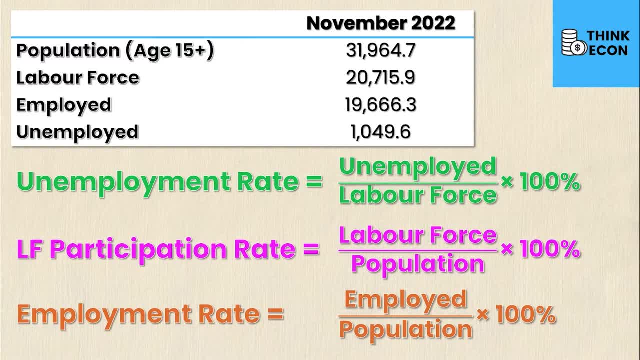 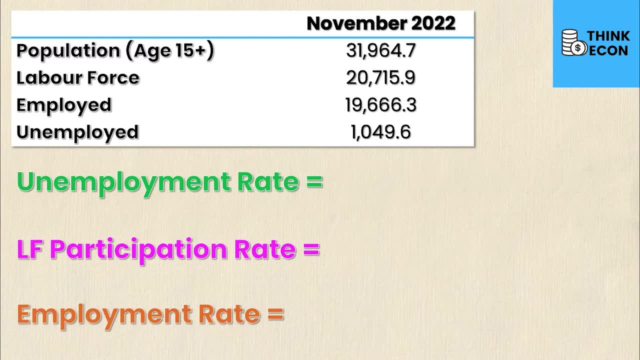 employment rate will not sum to one. I just wanted to make that distinction, because that's an area I see a lot of students mess up. So we have all of the information we need to calculate these. so let's get started. For the unemployment rate, we have the total number of people unemployed. 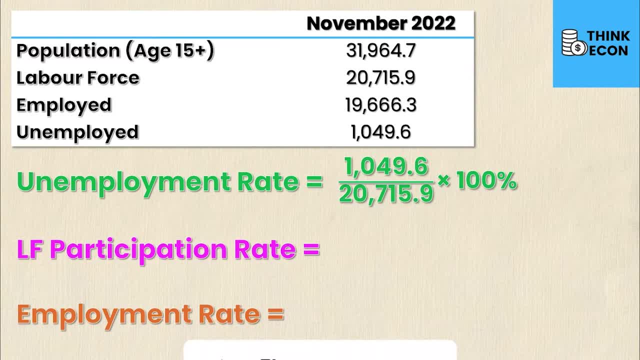 which is 1,049.6.. Remember, this is in terms of thousands divided by the total labor force, which is 20,715.9.. This gives me a decimal value of 0.0507.. And of course, I would multiply that. 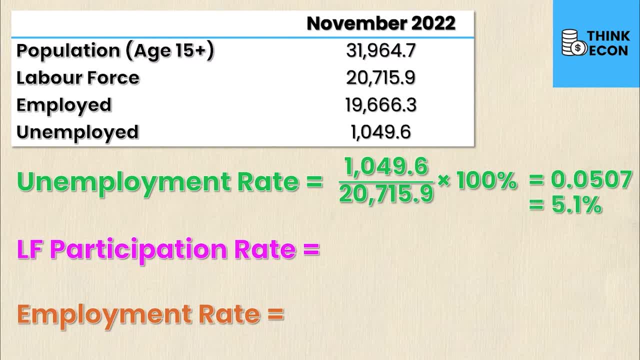 by 100%, because I want it as a percentage, and that gives me 5.1% For the labor force participation rate. I have my labor force, which is 20,715.9, divided by the total working age population, which is 31,964.7.. This is going to give me a decimal value of 0.6481,. 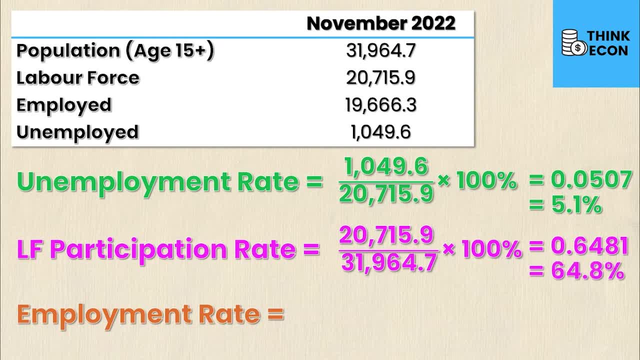 which, multiplied by 100, to turn it into a percentage, is going to give me 64.8%. Finally, we have the employment rate which, remember, is the number of people employed divided by the working age population. That gives me 19,666.3 divided by 31,964.7.. 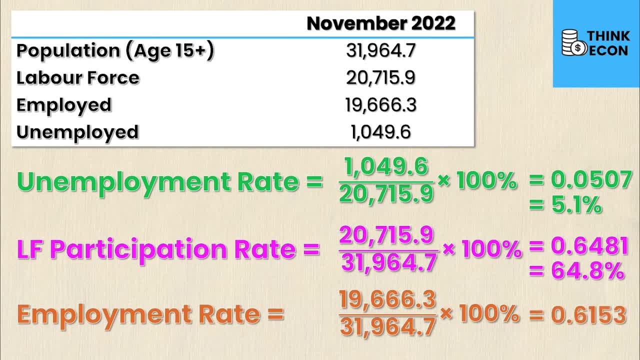 That gives me a decimal value of 0.6153.. And, of course, multiplying by 100 to get myself a percentage: 61.5%. Now going back and checking the labor force survey data, all three of these rates that you calculated perfectly match the. 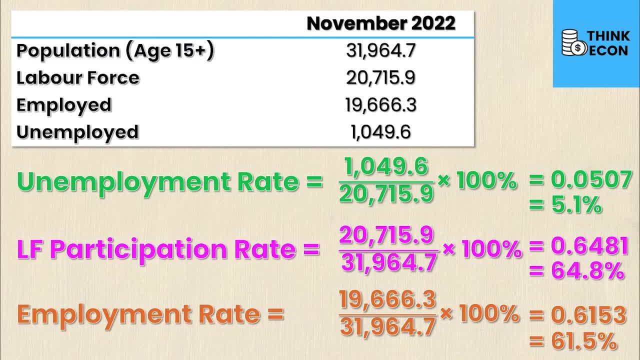 rates determined by the statistics Canada. And there you have it. It's as simple as that. Once again, remember that the denominator for the unemployment rate is not the same as the denominator for the employment rate. Again, that's the biggest mistake that students make. 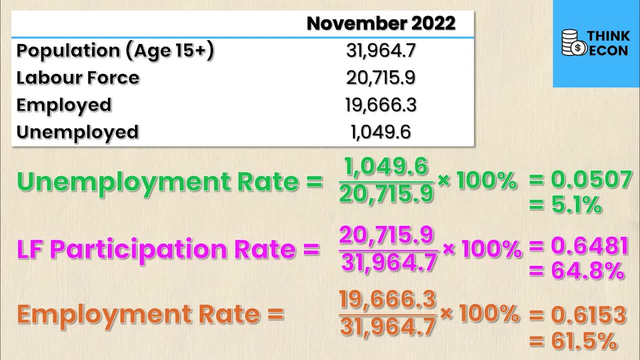 when calculating these rates And therefore the unemployment rate and the employment rate do not sum to 100%, as you can clearly see. In the future we plan on making a video where you're given the employment rate, the labor force participation rate and the employment rate.